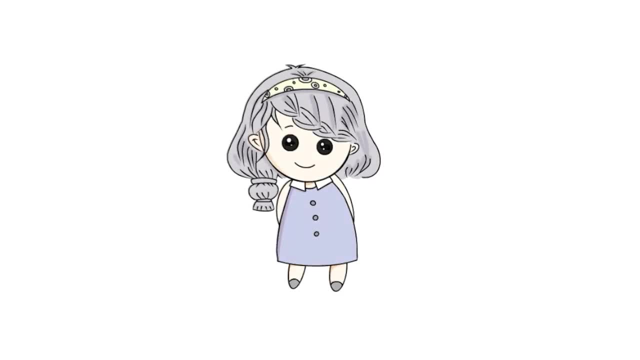 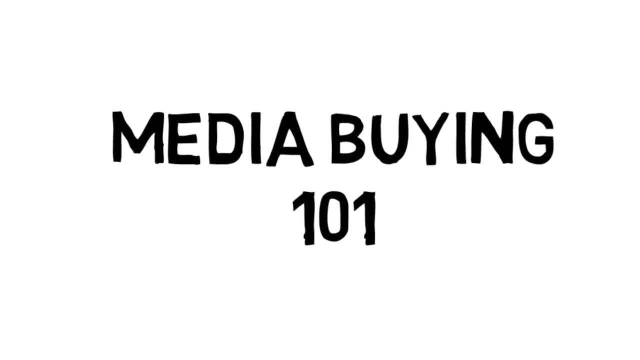 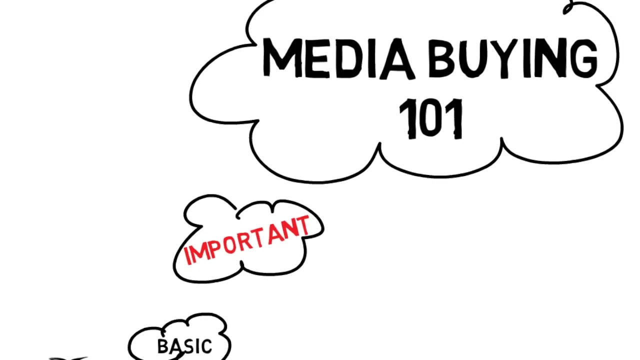 Hi everyone, it's Bailey here. Welcome to my channel. In today's video I want to talk about what is media buying? Media buying is a very, very basic and important concept in marketing, but I don't fully understand it until second year entering the workforce. 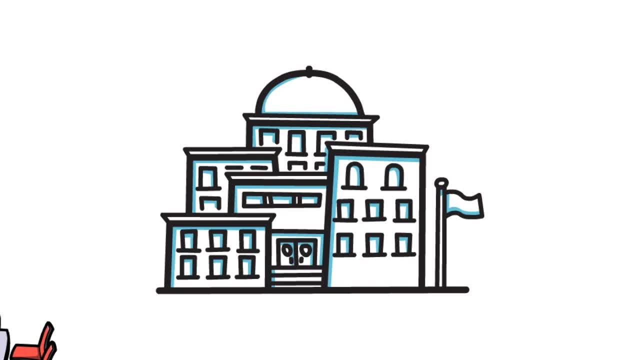 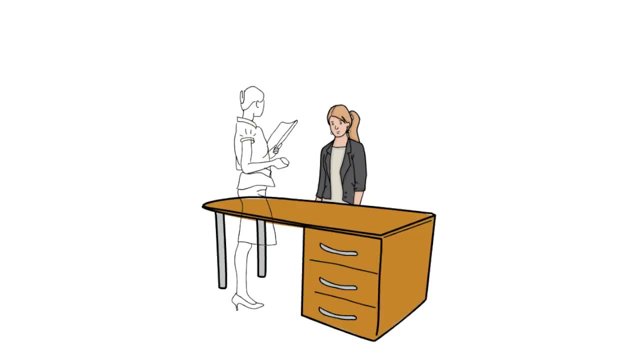 And I was a marketing major in college. You're probably thinking, Bailey, what are you doing for years in college? Yeah, I don't really know. I think the first time I heard of the term it was at a college career fair. At that time I was literally like: I want to do marketing. 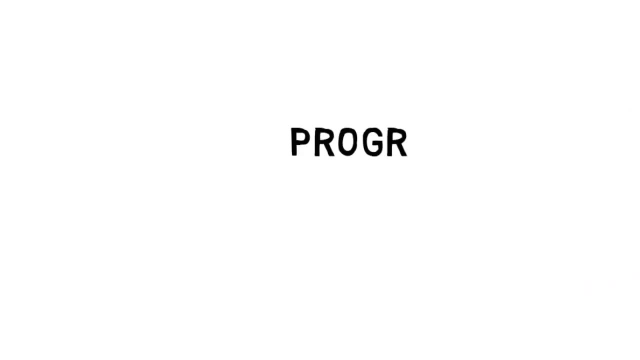 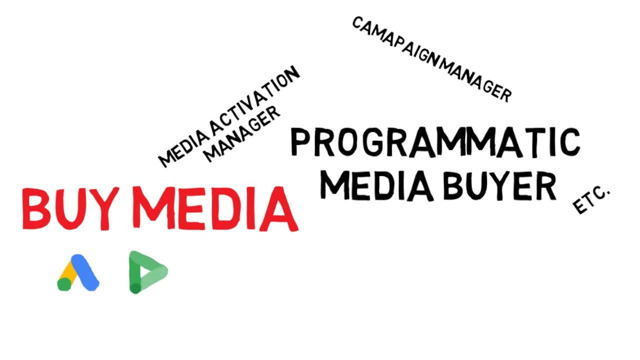 not media buying. I'm a programmatic media buyer now. Sometimes it's also called a campaign manager or a media activation manager or something else. The job scope might vary a bit, but the core function of the job is to buy media. If you are a current marketing student or a reason grad and you are 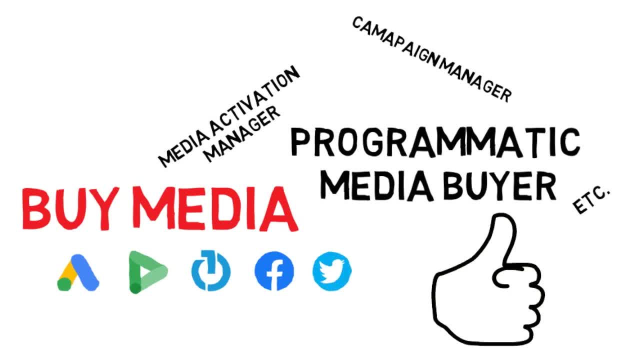 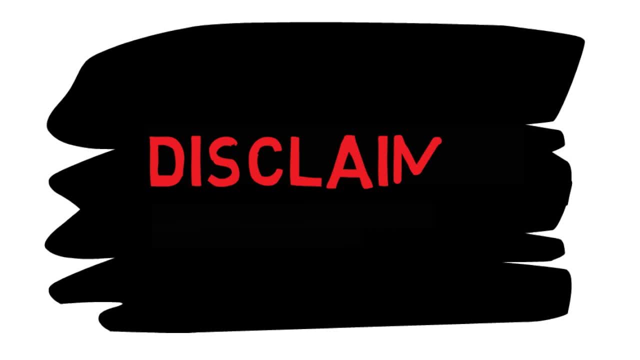 watching this video. I'm really proud of you for getting ahead of yourself. Before we start, I just want to make a disclaimer that all of the knowledge shared in this video it's solely based on my understanding of the industry and it only represents my personal opinions. Feel free to. 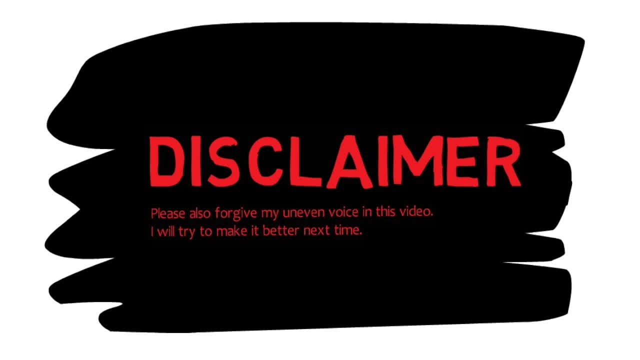 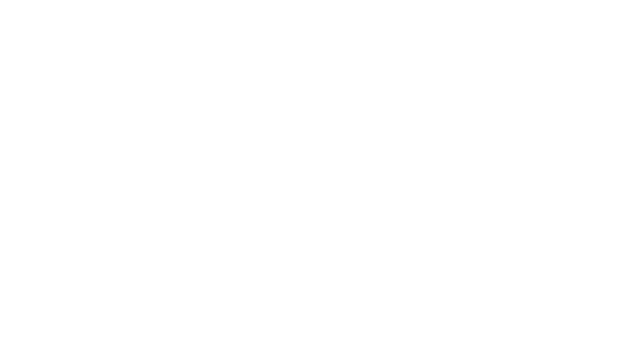 share your thoughts in the comments down below. I would love to hear from you. If you have any questions, let me know. in the comments, I also have listed some of the resources I used for this video in the description box. Alright, without further ado, let's get into it. What is media? 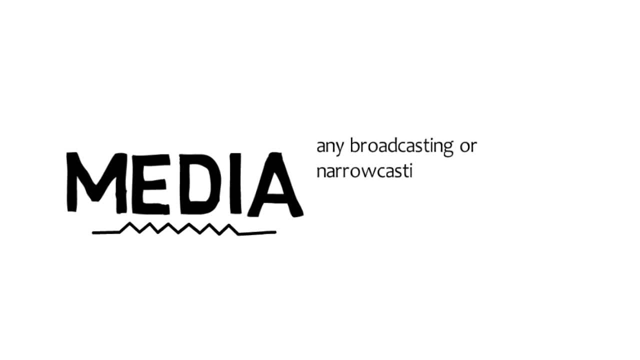 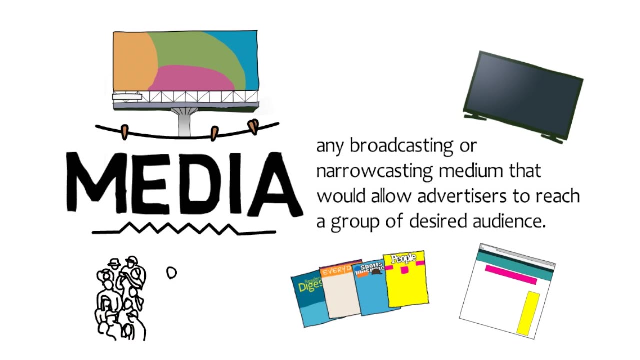 What would appear in your mind when hearing the word media In marketing? when we are talking about media, we are usually referring to any broadcasting or narrowcasting mediums, such as TVs, billboards or the internet that would allow us to reach a group of desired audience. 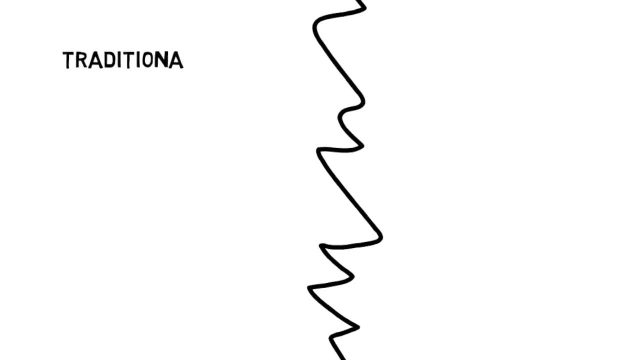 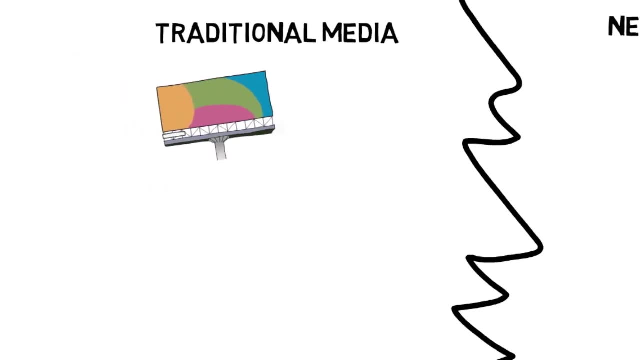 We tend to group all of the medias into two groups: offlines and onlines, or traditional and new medium. Traditional media includes mostly non-digital media channels such as billboards, radios, TV prints and more. They tend to be less measurable, more expensive. 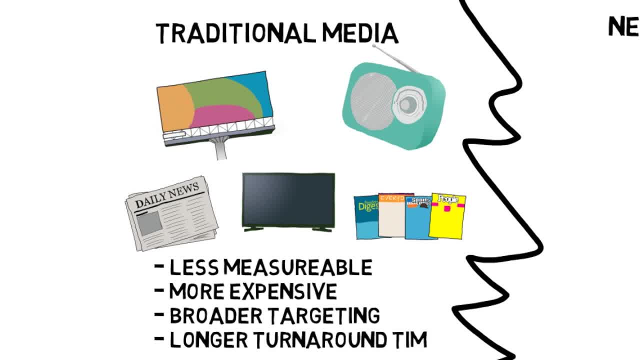 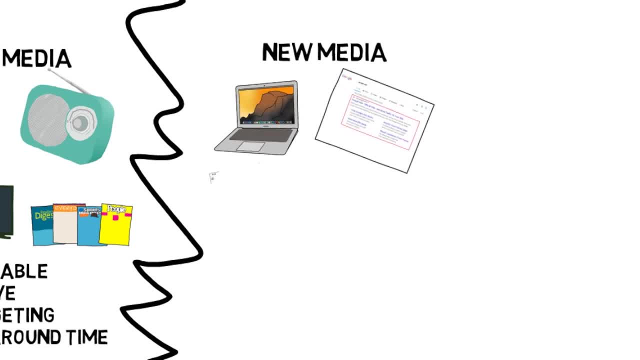 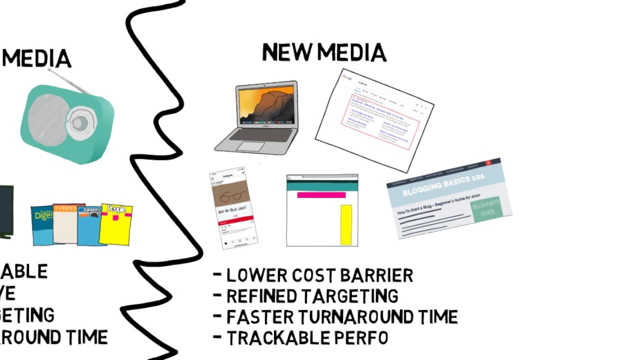 broader targeting and need longer turnaround time. New media includes mostly digital media channels such as SEM, social media, blogs, online news publishers, etc. Digital media has lower cost barriers, allows more refined targeting, faster turnaround time and, most importantly, 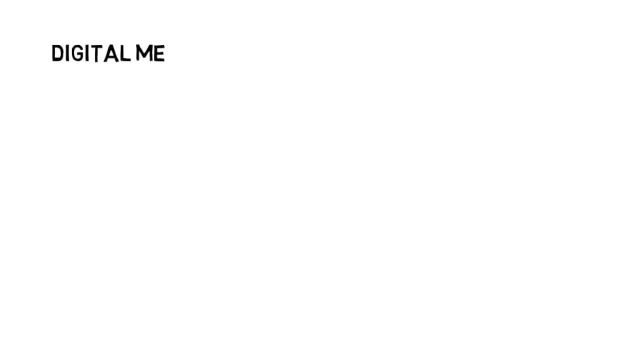 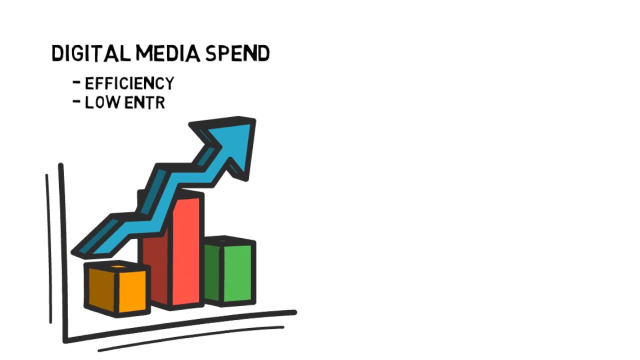 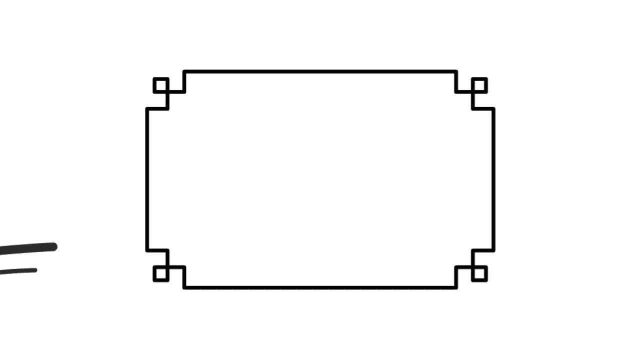 it's trackable. Over the last decades or so, these digital channels have gained their popularity in the advertising space due to their efficiencies and lower entry points. However, I'm not saying that we should stop buying traditional media. You should buy whatever media that's suitable for your. 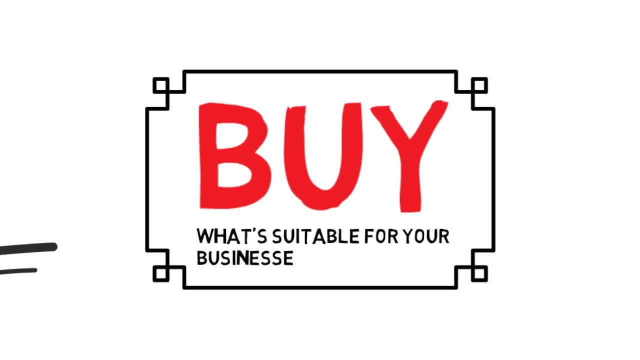 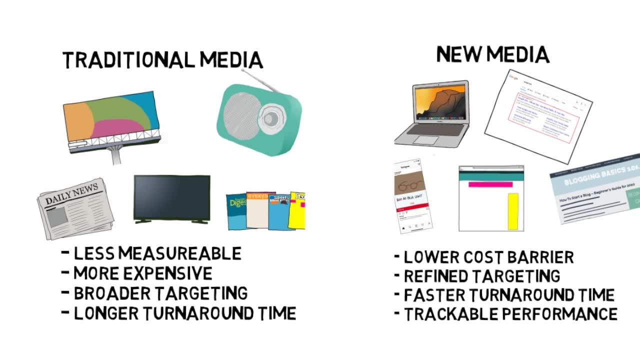 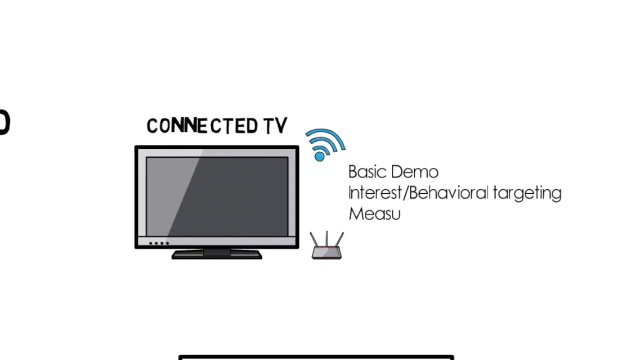 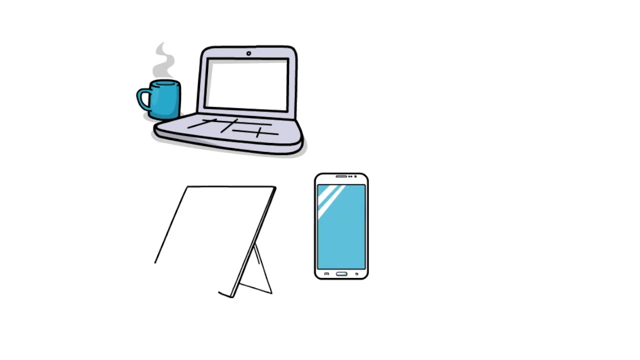 or your client's business goal. As our technology continues to advance, the line between traditional and new media would actually become blurry. For example, connected TV allows us to buy TV inventory programmatically and with refined targeting ability. In the future, what we consider as new media today would also become old media. What I like 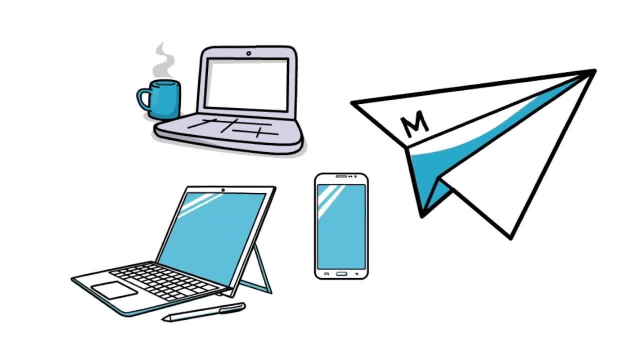 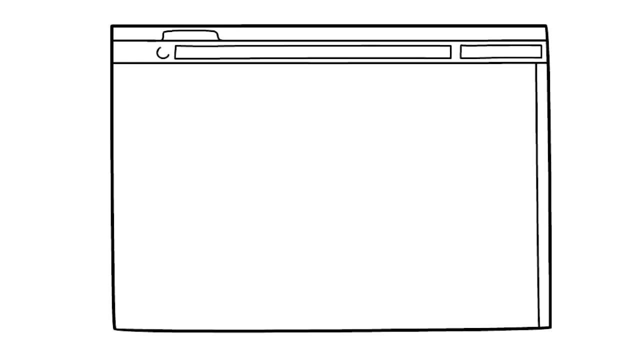 about my job is that it's always evolving. I consider it to be at the frontier of tech and marketing. Now that we have a better understanding of what is media, we can talk about what is media buying. When we are buying media, we are actually buying the opportunity to. 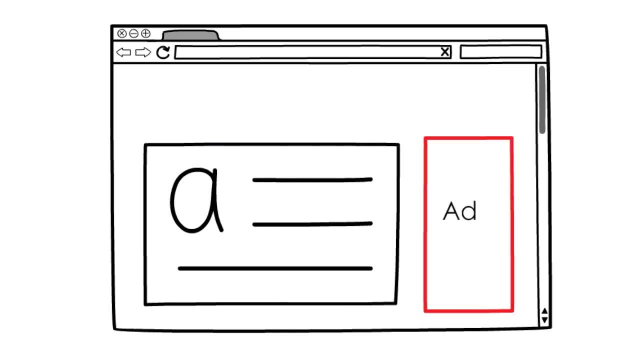 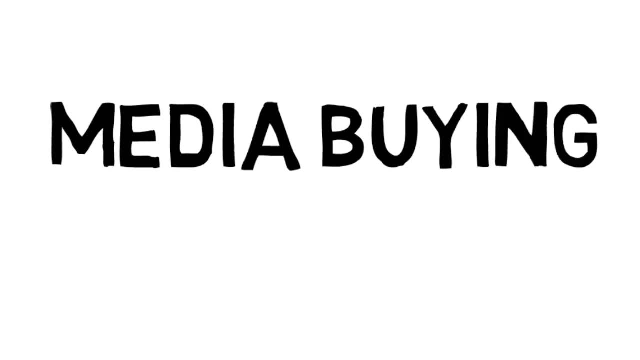 show our ads around any desired content time. when I have to explain my job to someone who have no marketing backgrounds, I tend to just simply tell them that I place ads online. However, media buying is much more than that, especially for digital media. Media buying is the purchase of advertising inventory from any media channels. 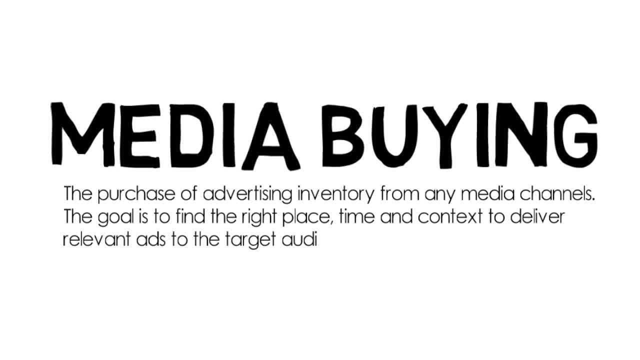 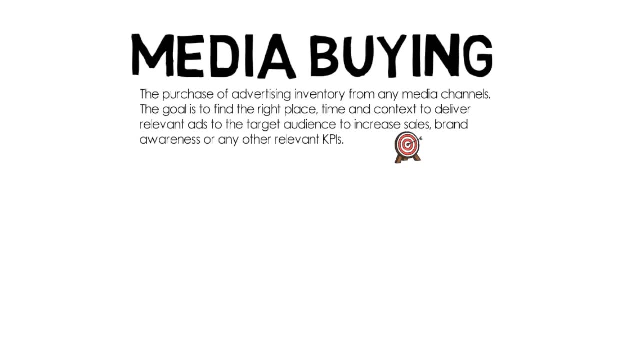 that we have previously mentioned it. The goal is to find the right place, time and context to deliver relevant ads to targeted audience, to increase sales, brand awareness or any other relevant KPIs. There are two ways to buy media from publishers or platforms: Direct buy usually.